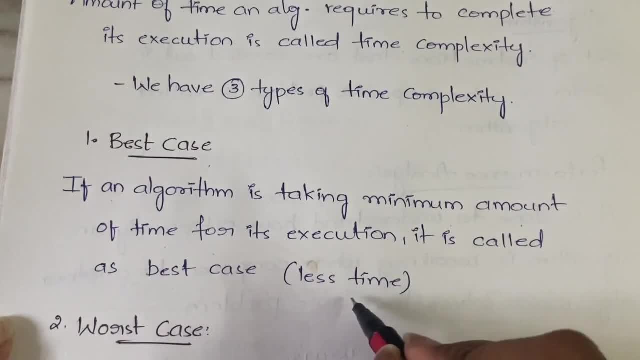 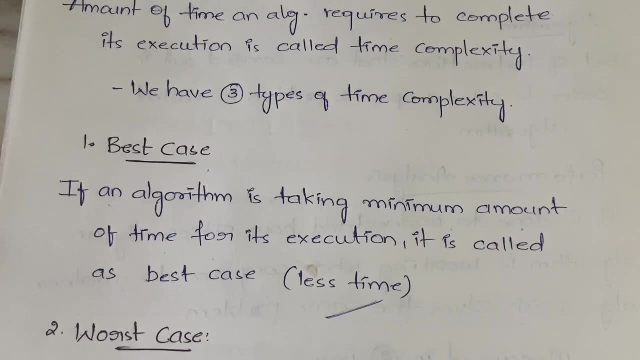 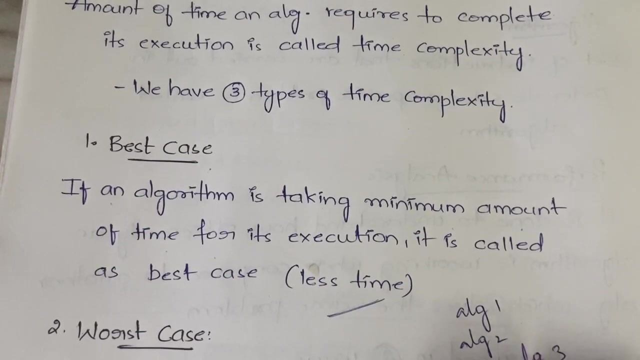 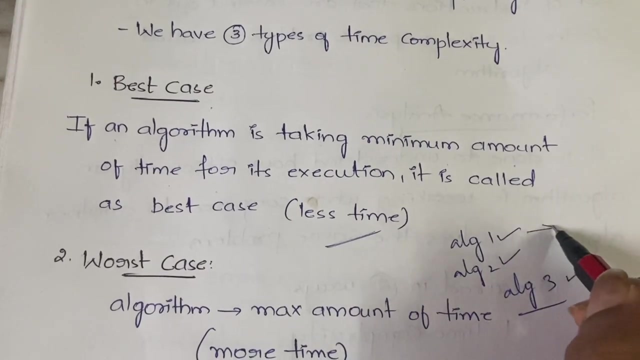 then it is called as best case time complexity. That is, if it is taking less amount of time, then it is called best case time complexity. Okay, in general, in general, to be more clear, suppose you have an algorithm one, algorithm two and algorithm three. all the three algorithms are designed for the same purpose. This is for adding, this is for adding and this is also for adding. Now, this algorithm one is taking only two seconds to perform the addition. Algorithm two is taking 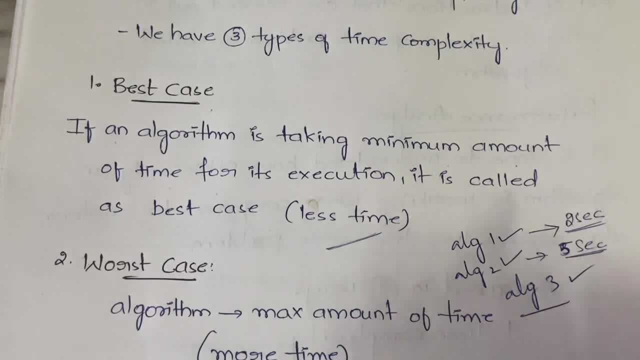 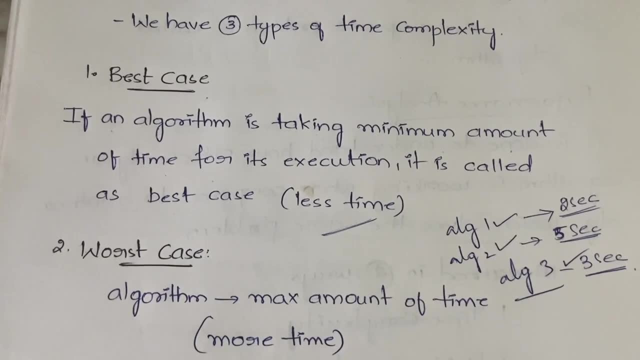 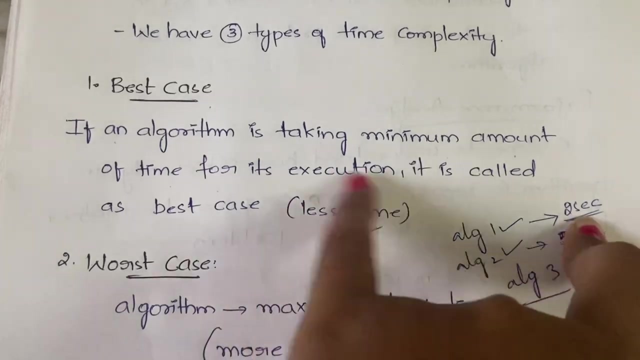 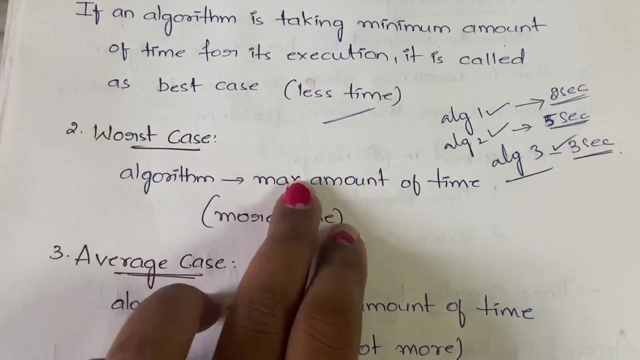 five seconds. let us take five seconds of time to perform the addition. Algorithm three is taking some three seconds of time. Okay, Now, among these three algorithms, which is taking the minimum amount of time, that is, less amount of time? the first one. So this will come under the best case, that is, it has to take minimum amount of time. Okay, Next comes the worst case. Worst case means it has to take maximum. So if an algorithm is taking maximum amount of time to complete its execution, 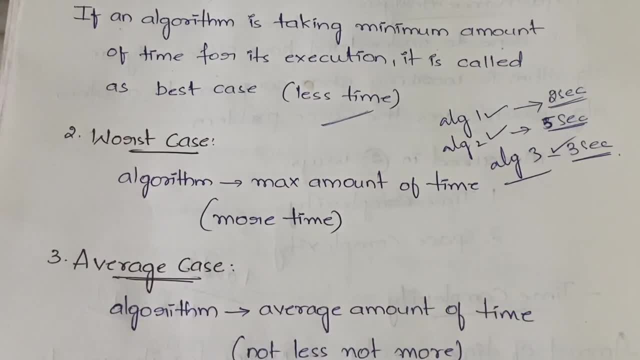 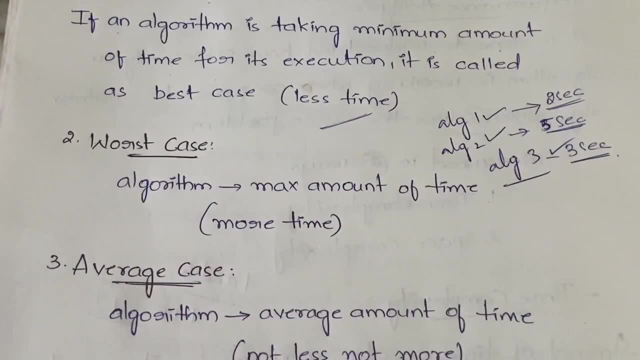 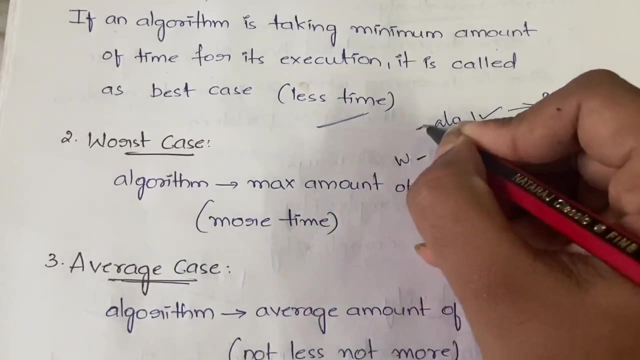 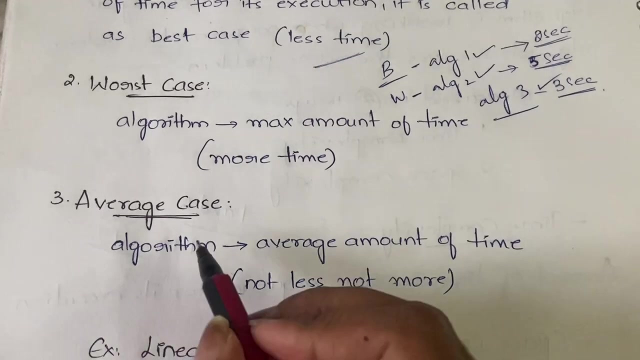 then it is called as the worst case that it is taking more amount of time. For example, here, among these three algorithms, which is taking maximum amount of time? five seconds, algorithm two is taking right. So this will come under the worst case, this will come under the best case. Are you? are you guys getting it Next average case. So average case if an algorithm is taking average amount of time that is not less, not more. See here three. 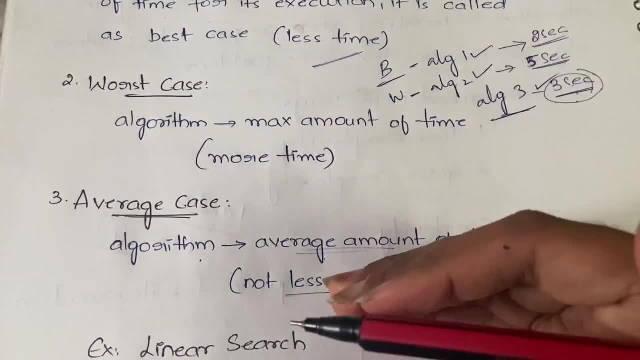 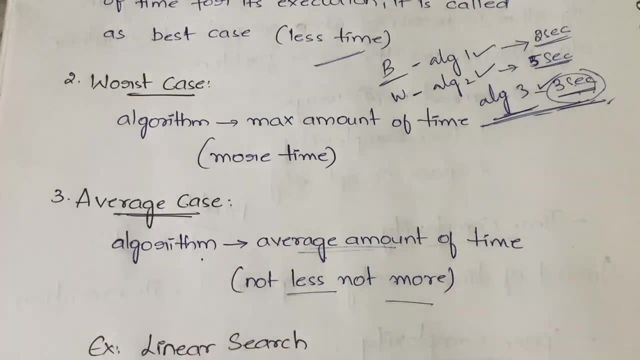 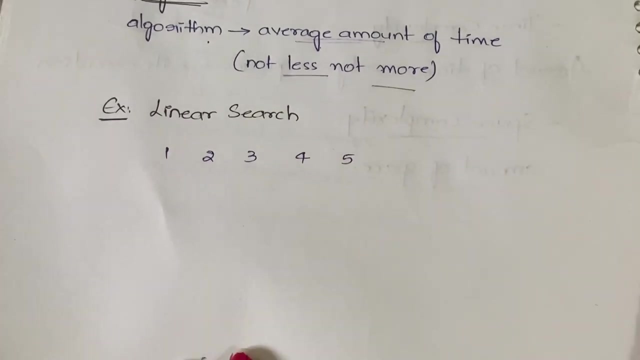 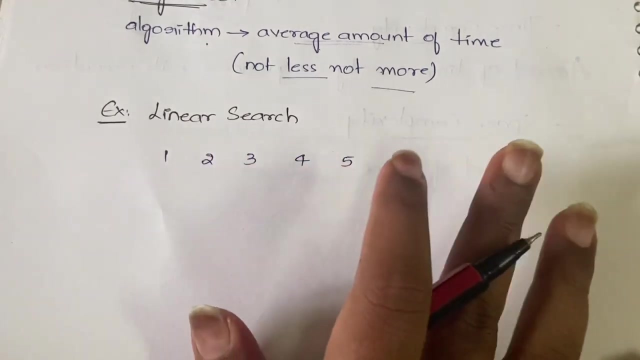 seconds we have for algorithm three. three is not a minimum one, not the maximum one as well, So that is why we take it as a average case. time complexity. Okay, Now let us take an example with linear search. So you, I guess you already know what is linear search. If no, no issues, I'll explain you. For example, you are having 12345, right, Suppose, if you want to search for a number four, okay, in linear search. 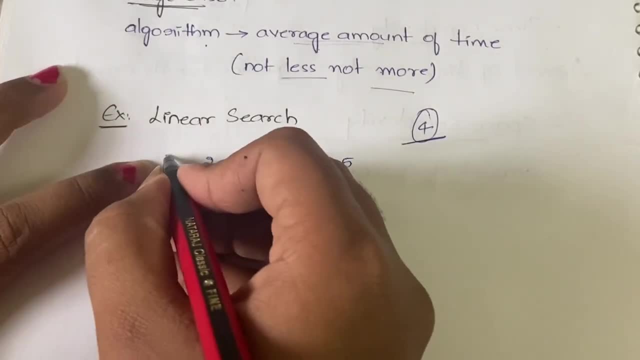 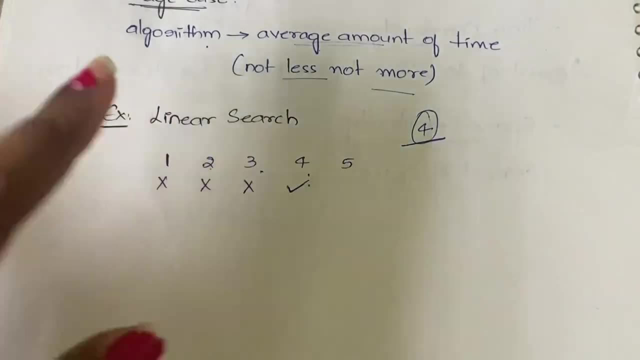 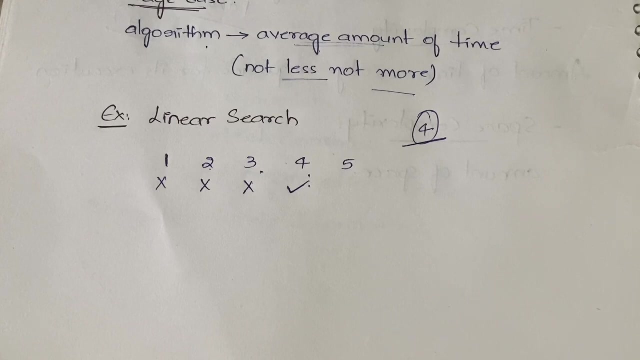 what you'll do is one by one. you'll search First, you'll search with the first element. Is it matching No Second element matching No Third element? matching No Fourth element? Yes, it is matching. So you will be searching element by element. Got it In binary search. what you do in binary search- and there are some other searching algorithms, right In that you will not do this one by one, you will not search. But in case of this linear search, you will be searching element one by one. This is linear search. Okay Now. 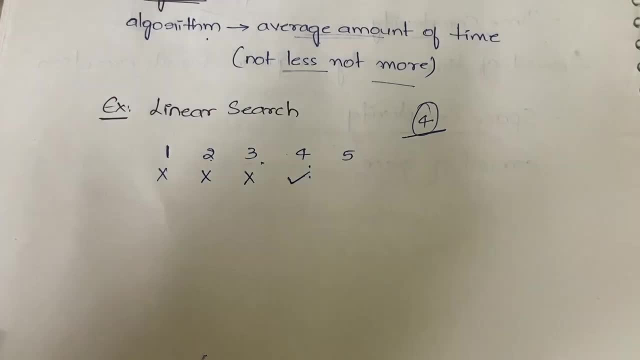 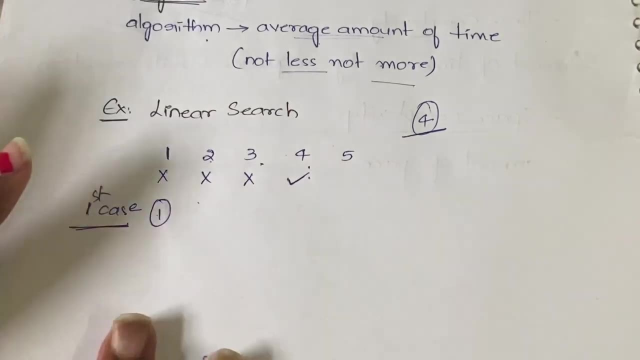 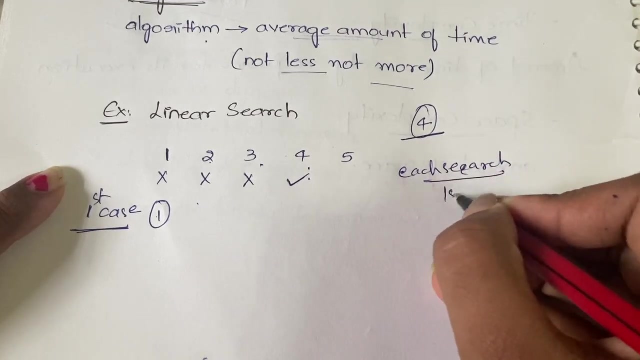 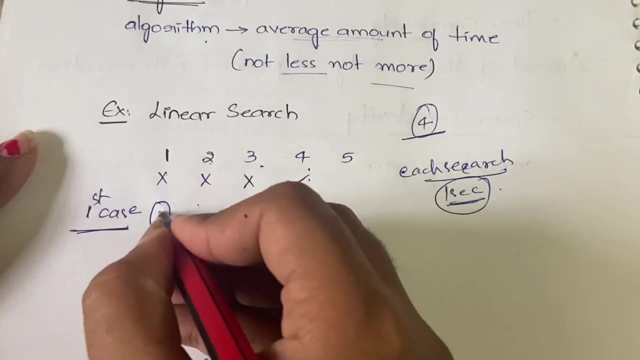 let us relate it with our time complexity First. first case: suppose you are searching for element one. Okay, For each search, let us take: we need one second of time. one second of time for each search. it is taking one second of time. Now you're searching with one right, You're searching for one and you found it in the first place itself. That is how much time you're taking for this. 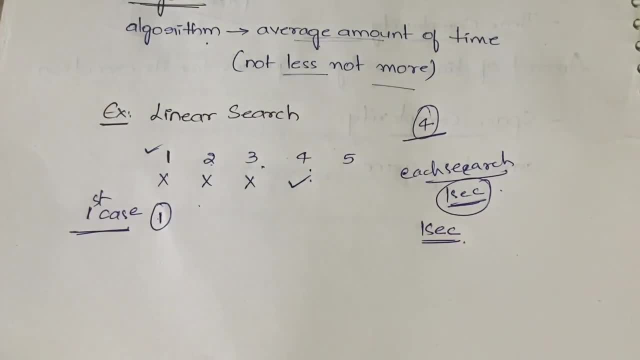 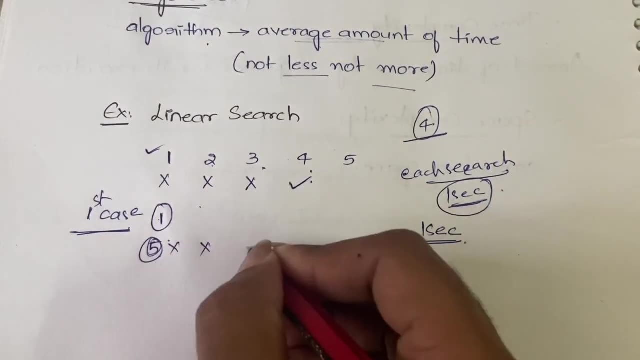 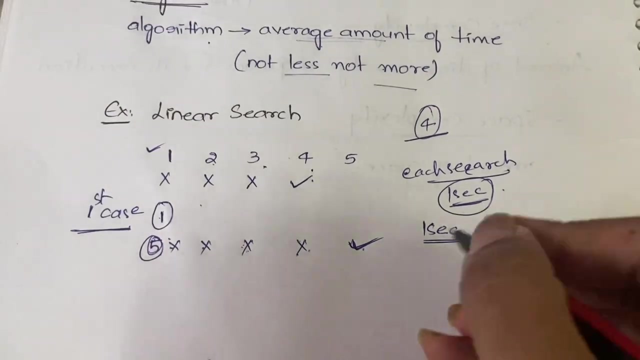 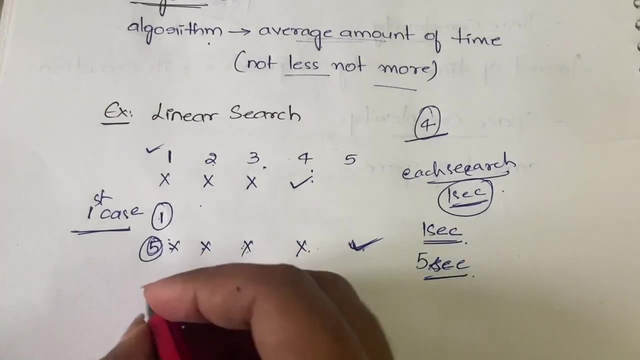 you're taking only one second of time, right. And next, if you want to search for element five, okay, element five is not present here. it is not present here. it is not present here, it is not present here, but it is present here. that is 12345 total five seconds of time you're taking in order to search for element five. Okay, suppose you want element three. So for element three, it is not present here, it is not here, but it is here for this. 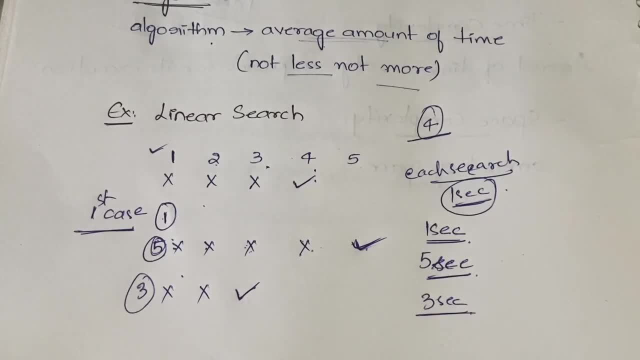 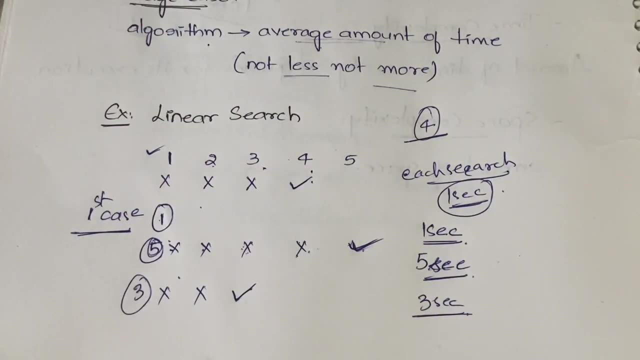 it is taking three seconds of time. ok, now, what is the best case? time complexity, first one, because it is taking only one second. in the first attempt itself, you are getting the desired number. ok, now 5 will come under the worst case. why? because it is taking more amount. 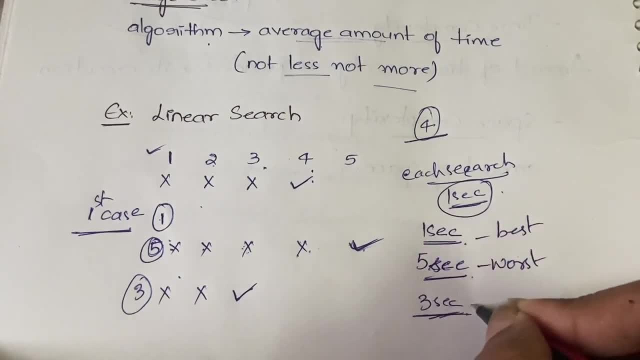 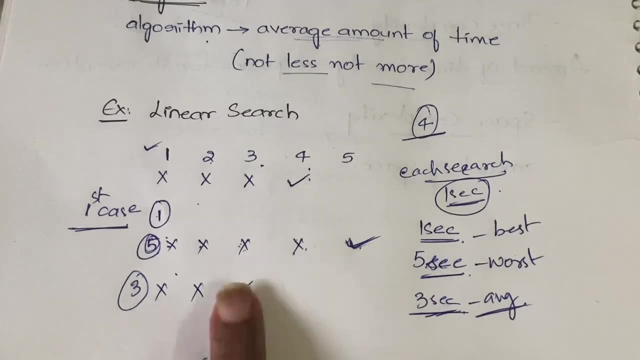 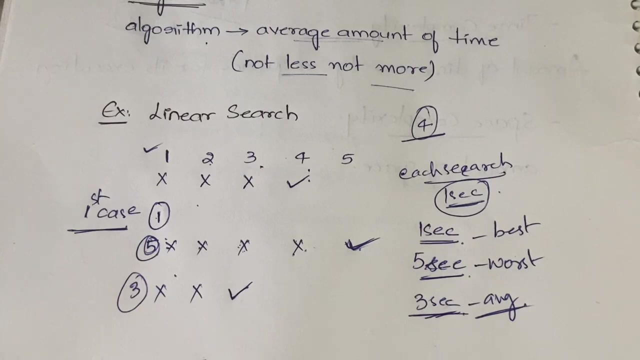 of time. ok, this will come under the best case. 3 will come under the average case. time complexity- why it is taking a average amount of time. ok, that is only 3 seconds. it is not minimum, not maximum, ok, so this is about time complexity, guys. very, very simple. ok, if it is taking maximum.